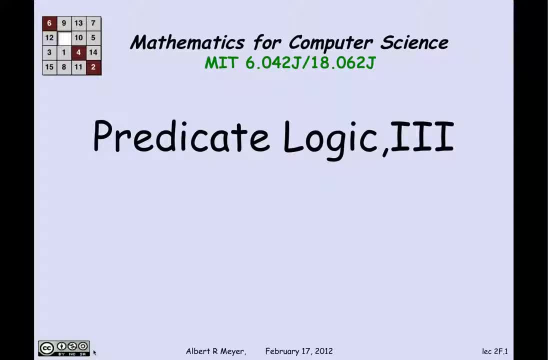 In this final segment on predicate logic, there are two issues that I'm going to talk about. The first is some problems with translating AE quantifiers and EA quantifiers into English, or rather from English into logic. We've seen examples in class that English is ambiguous. 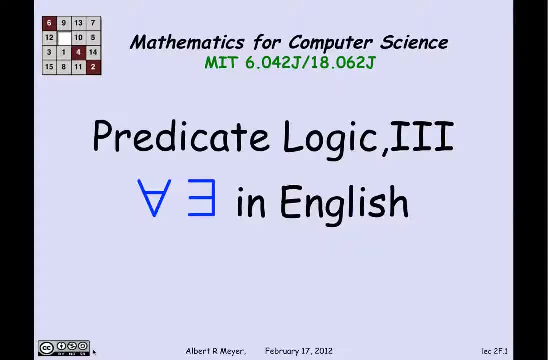 and I want to show you two that are, I think, interesting and provocative, just as a warning that translation is not always routine. And then the second topic is an optional one, just to kind of make some comments about the amazing results in metamathematics. 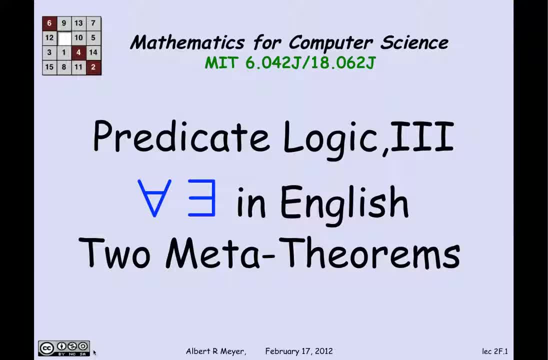 the mathematics of mathematics, or more precisely the mathematics of mathematical logic, and two fundamental theorems about properties of predicate calculus which go beyond this class and are optional. I would suggest that you take a look at the next slide. It's worth listening to the AE in English example and if you want to skip the short discussion. 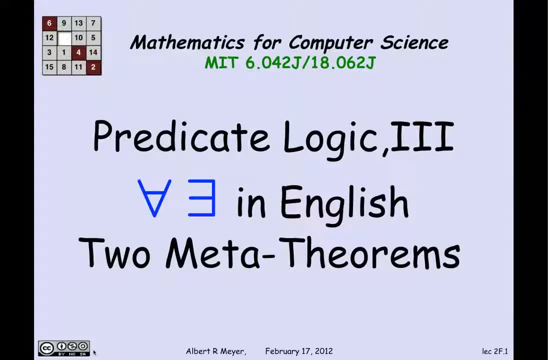 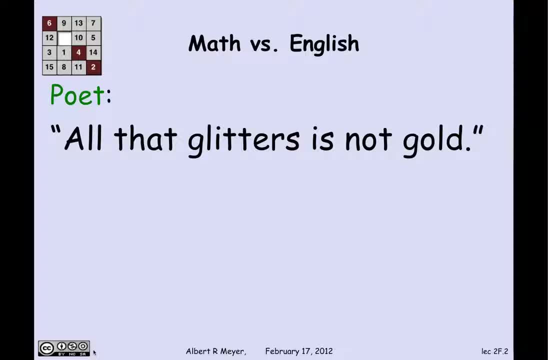 of the metatheraums. that's fine, because it's never going to come up again in this class. Okay, so let's look at this phrase in English where the poet says: all that glitters is not gold. Well, a literal translation of that would be that if we let G be, glitters 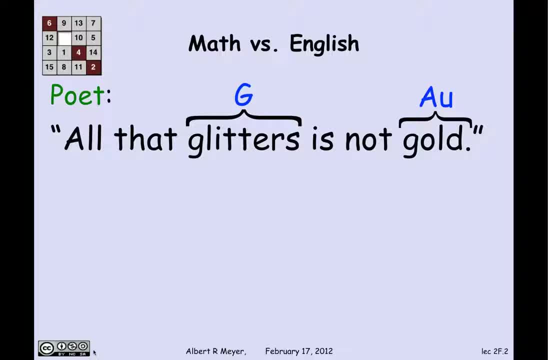 and I can't use G again. so we'll say: AU is gold. then this, translated literally, would say: for every X, G of X. if X is gold implies that not gold of X. All right, so is that a sensible translation? 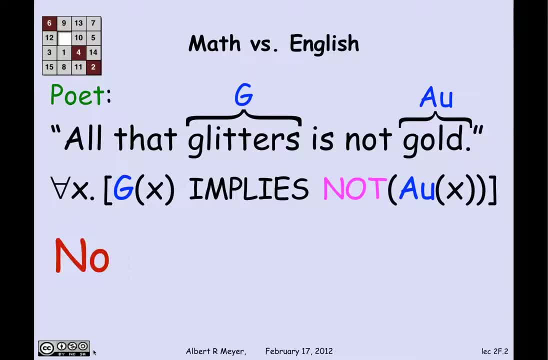 Well, it's clearly false, because gold glitters like gold and you can't say that gold is not gold. So this is not what's meant. It's not a good translation, It doesn't make sense. Well, what is meant? 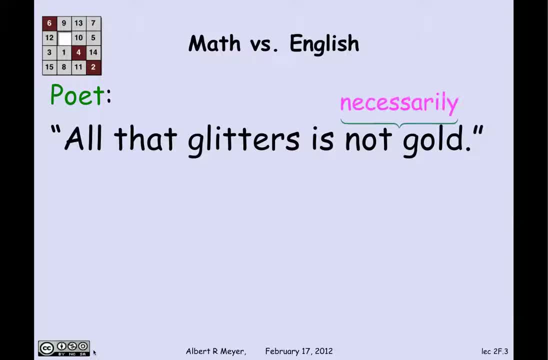 Well, when the poet says all that glitters is not gold, he's really leaving out a key word to be understood from context: All that glitters is not necessarily gold. He's using poetic license. You're supposed to fill in and understand his meaning. 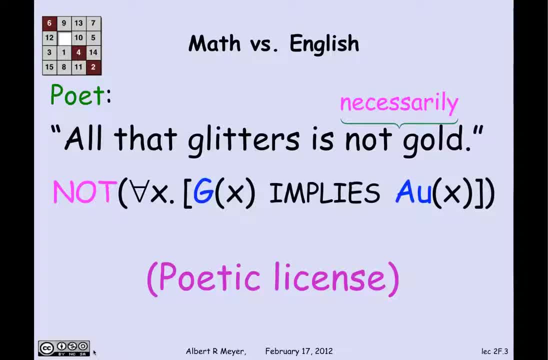 And the proper translation would be that it is not true that everything that glitters is gold. It is not the case that for all X, if X glitters, then X is gold. So it's just an example where a literal translation, without thinking about what the sentence means. 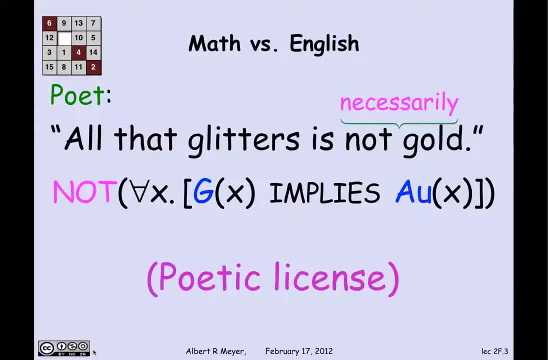 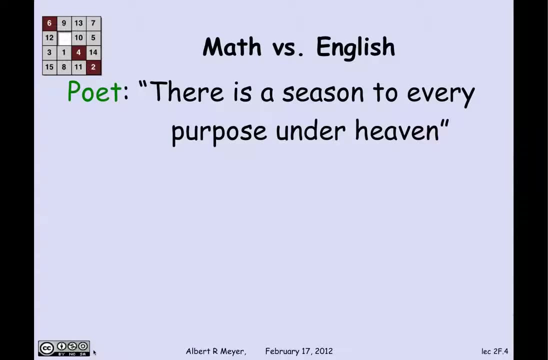 and what the poet who articulated the sentence intended will get you something that's nonsense. It's one of the problems with machine translation from natural language into precise formal language. Okay, let's look at another example. The poet says: this time there is a season to every purpose under heaven. 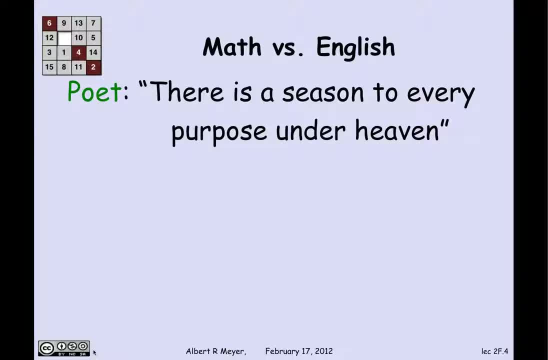 This is a variant of a biblical phrase. So what does it mean? Well, the literal translation would be: there exists an S that's a season, such that for every P that's a purpose, S is for P. Well, that, from the way that quantifiers work. 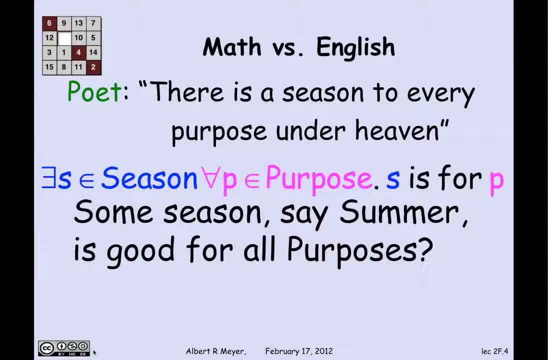 means that there's some season, Say summer, that's supposed to be good for all purposes. Well, that's not right, because summer's not good for snow shoveling, And if your purpose is to shovel snow, then summer will not do for you as a season. 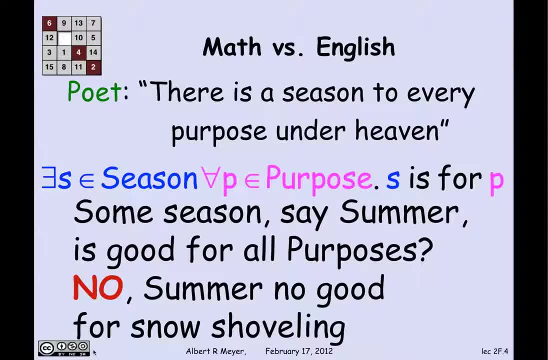 So even though it's phrased there is a season to every purpose under heaven, it's not the case that the intended translation is there is a season for every purpose. In fact, the poet really means to flip the quantifiers. 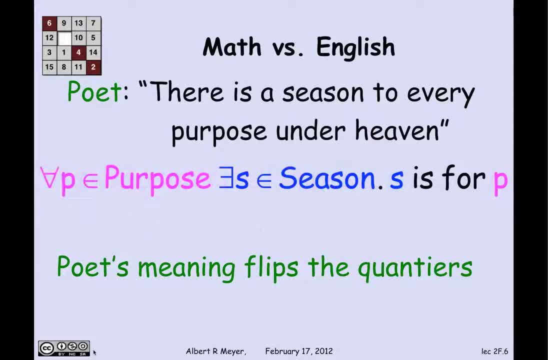 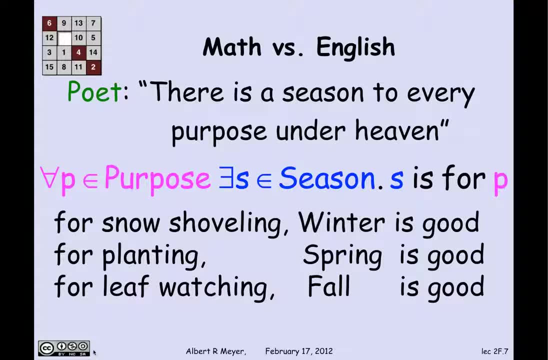 Which is what's shown here. We're going to switch them around so that we are really saying: for every purpose there is a season such that S is for P, For snow shoveling, winter's good, For planting, spring is good. 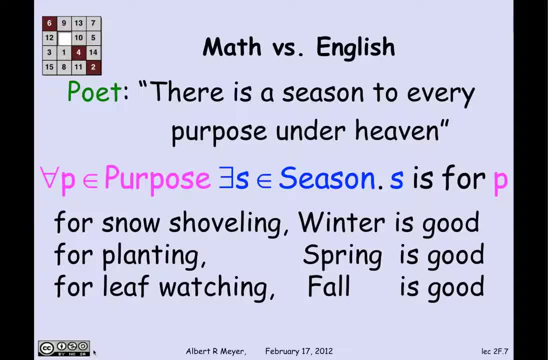 For leaf watching, fall is good, And that is in fact the intended translation here, Although I remind you that there's a famous historical man, Sir Thomas More, who was described as a man for all seasons. That would be a case where there was man, one man, who was good for all seasons. 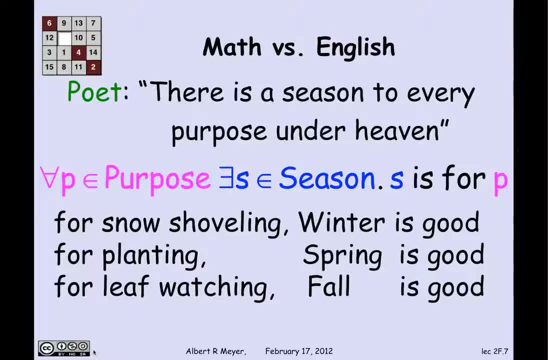 He was a polymath, a writer, a, a cleric and the Chancellor of England for many years, until he had a falling out with Henry VIII which served him ill. Okay, that's the end of those two examples, whose point is just to warn you that translation from: 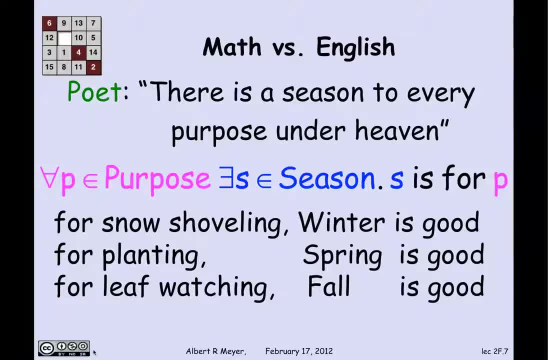 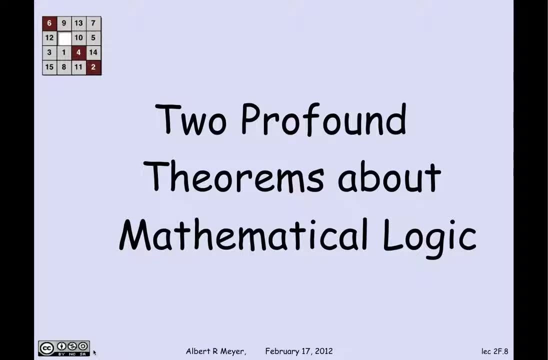 English into math is not something that can be done in a mindless mechanical way. Sometimes the quantifiers really are meant to go the other way from the way that they literally appear. Now we're going to shift to another topic, which is just two profound theorems from mathematical logic. 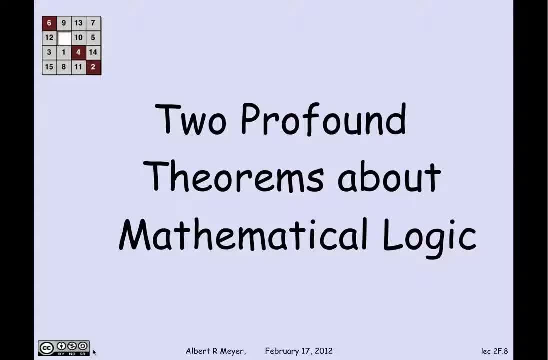 about the properties of predicate calculus that are worth knowing about and that describes the power and limits of logic. So these are called meta theorems because they're theorems about theorems. They're theorems about systems for proving theorems. 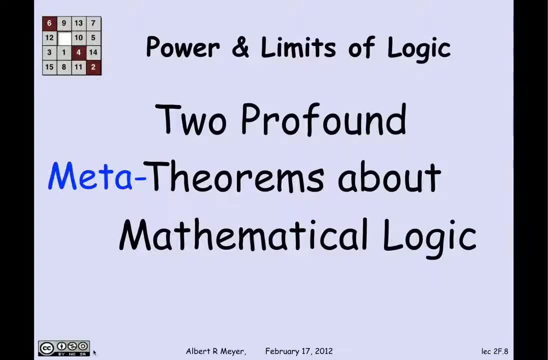 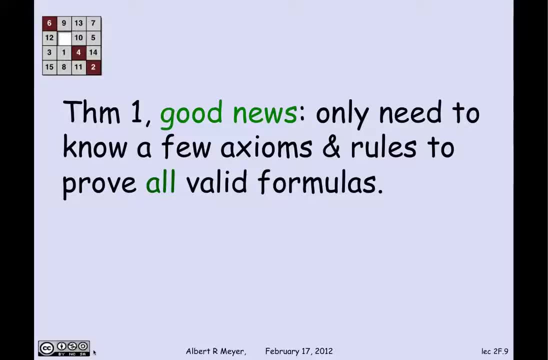 And that phrase meta means going up a level. So the first theorem is a good news theorem. It says that if you want to be able to prove every valid assertion of predicate calculus, there really is only a few axioms and rules that will do the job. 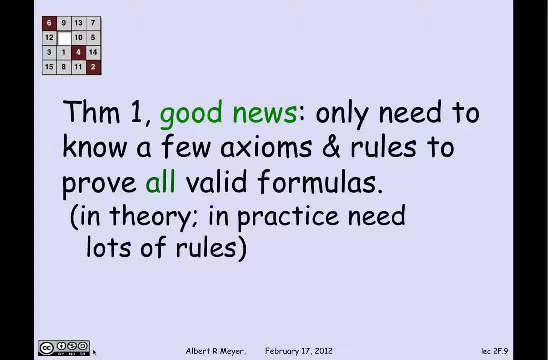 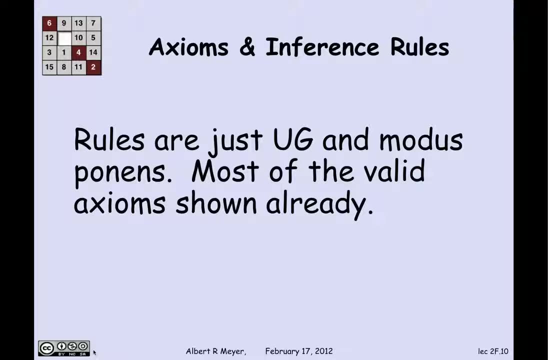 As a matter of fact, the rules that you need are just rules that you've seen already, namely modus ponens and universal generalization and a few valid axioms, which we've seen already. Let's go back a little bit. So there's a little mark here that says that, in practice, 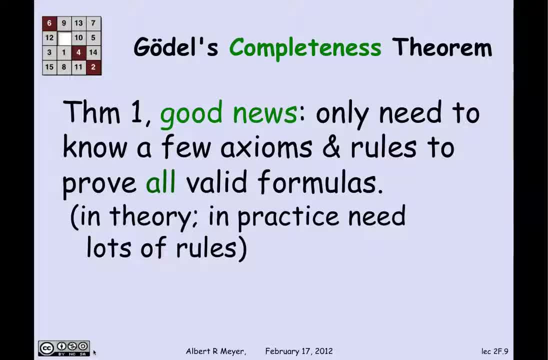 if you're really going to try to do automatic theorem proving, you need much more than this minimal system. But it's intellectually Interesting and satisfying that a fairly economical set of axioms and inference rules are in theory sufficient to prove every logically valid sentence. 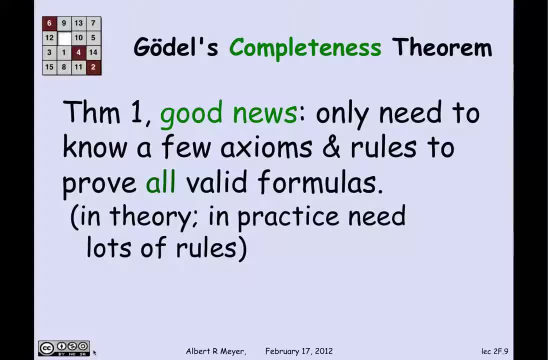 This is known as Gödel's Completeness Theorem. Gödel was the great mathematician, German mathematician, who spent the latter part of his life at the Institute for Advanced Study in Princeton as an emigre, And he has two matrices.